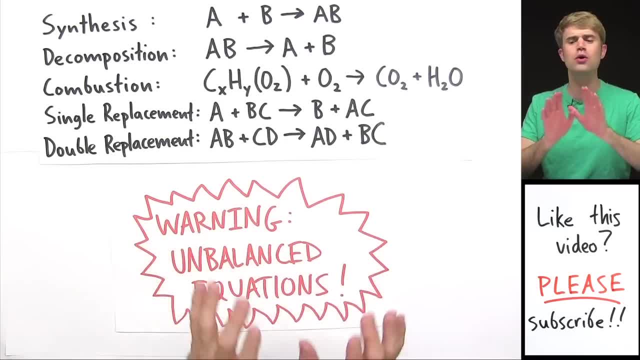 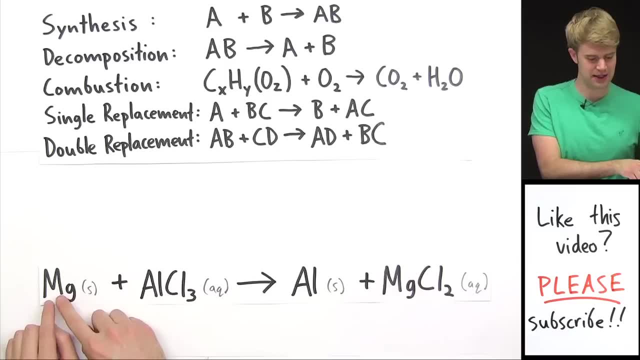 I just want you to focus on the elements and how they're rearranging, and I don't want you to worry about getting distracted by the coefficients. Okay, so let's start classifying reactions. Here's our first: Magnesium and aluminum chloride. give us aluminum and magnesium chloride. So what's? 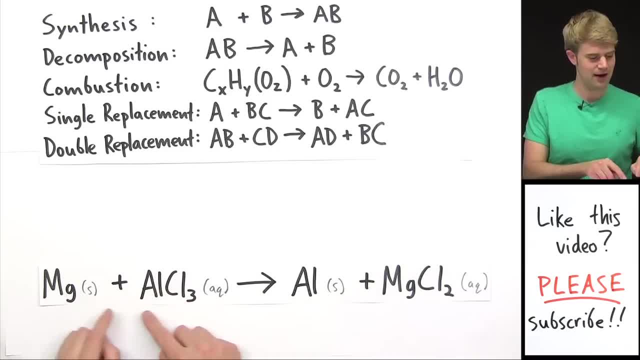 happening here. We have aluminum and chloride paired up here. Magnesium is on its own, and then magnesium comes and takes the place of aluminum. magnesium pairs up with chloride and kicks aluminum out. So when something like this happens, we're talking about a single replacement, also known as a single displacement reaction- C8H18. 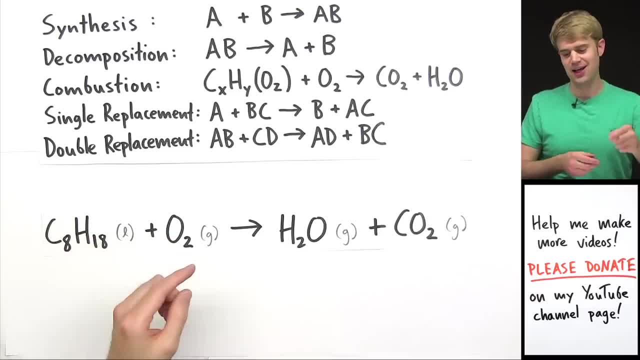 which is the chemical formula for octane, and oxygen gives us water, H2O and CO2.. So whenever we have something with carbon and hydrogen and we add oxygen to it and we get water and carbon dioxide, that is a combustion reaction, So this should. 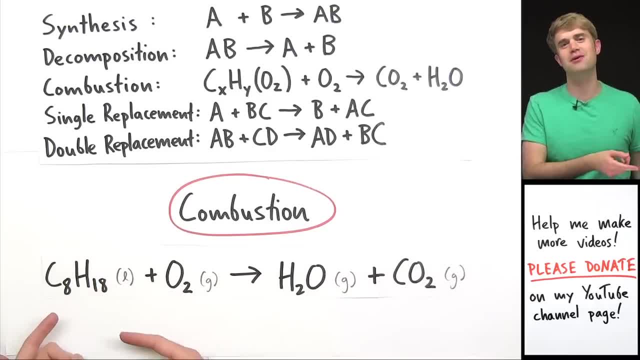 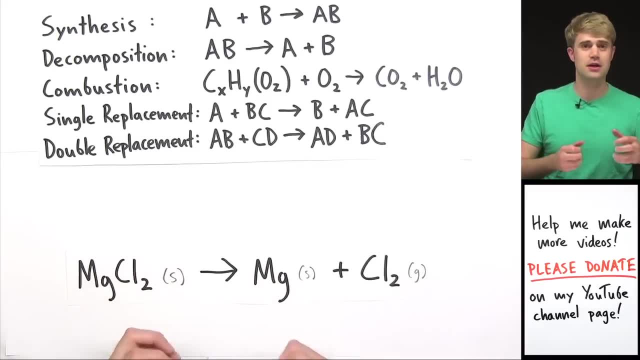 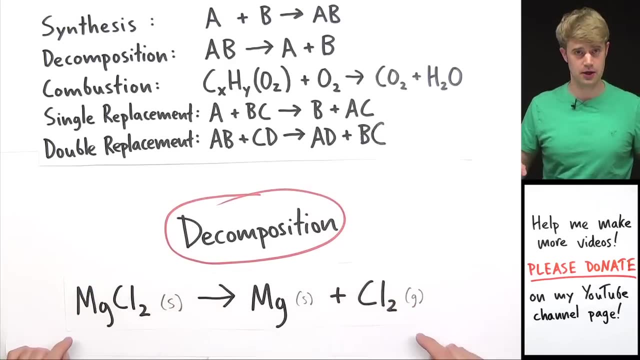 show us the combustion of octane, which is one of the components of gasoline. Magnesium chloride turns to magnesium and chlorine gas. What's happening here is a compound is breaking down into simpler components. This is a great example of a decomposition reaction: Magnesium and oxygen. 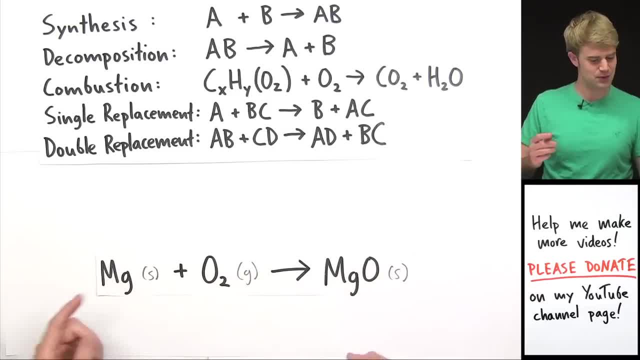 combine to give magnesium oxide. So what we have here is we have two simple things coming together to make something more complex, which is what happens when we have two things coming together. This is a synthesis reaction. So this is a synthesis of magnesium oxide. Now, just real quick. 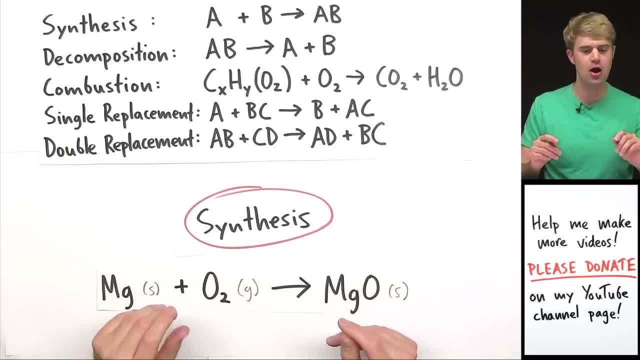 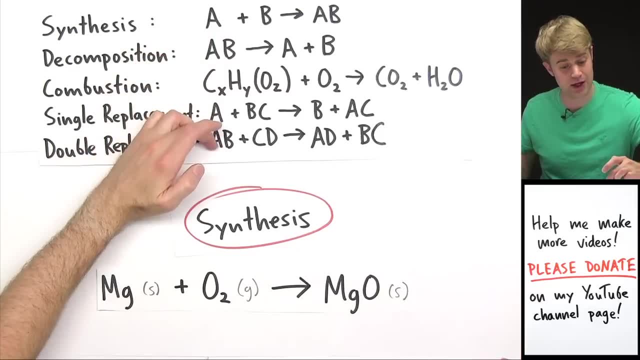 I'm referring to this chart to help classify the reactions, but chances are you wouldn't be allowed to use one like this on a quiz or a test. Okay, so just make sure that you really learn these sample equations for each reaction so that you're totally good with this when you run into it. 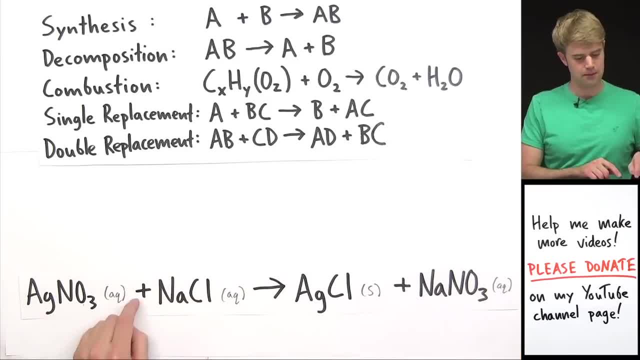 on an exam or something: Silver nitrate plus sodium chloride. give us silver chloride and sodium nitrate. What's going on here? Well, we have two pairs that then switch their partners. Silver was initially paired up with nitrate, and then silver ends up pairing up with chloride over. 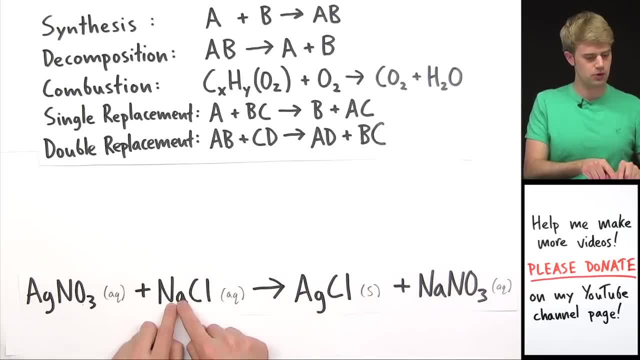 here, and sodium was initially paired up with chloride and then sodium ends and switches up here with nitrate. So this, where we have two pairs switching partners, is a really good example of a double replacement reaction. Sodium carbonate turns into sodium oxide and carbon dioxide. 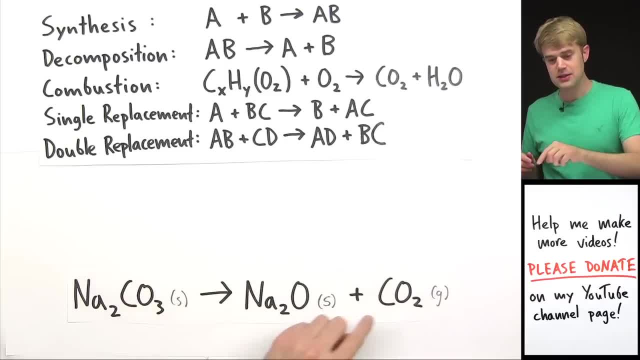 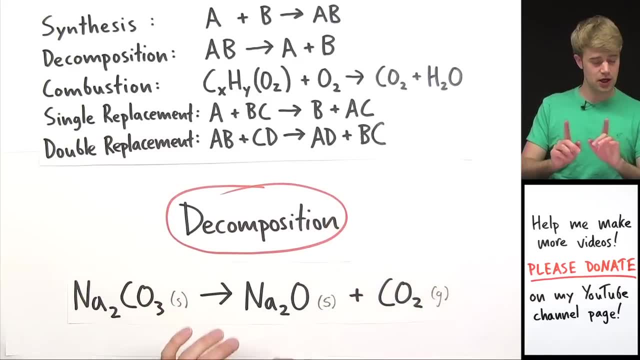 So here we have a compound breaking down into simpler compounds. This is what happens in a decomposition reaction. Now, in this decomposition reaction, we don't see this compound breaking all the way down to the elements that make it up. We're not getting just sodium, carbon and oxygen, but it's breaking down into simpler 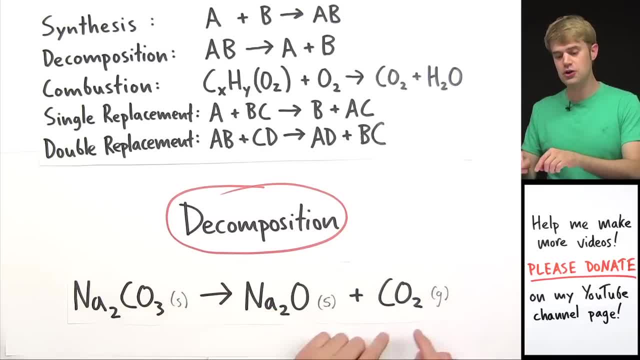 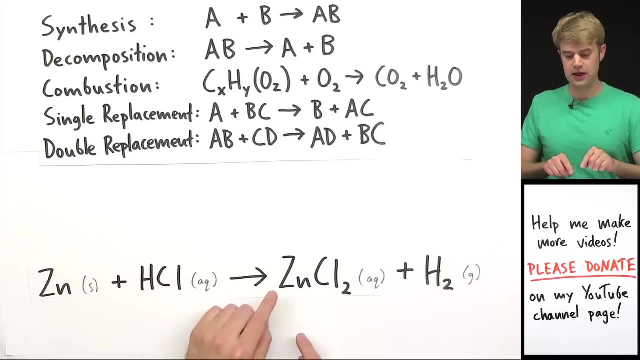 compounds that themselves are still combinations of more than one element. But that's okay. It's still a decomposition reaction just as long as we have something complex breaking into simpler pieces. Zinc by itself and HCl, which is called hydrochloric acid, give us zinc chloride and hydrogen gas. So what's happening here? Well, look at what's paired up. 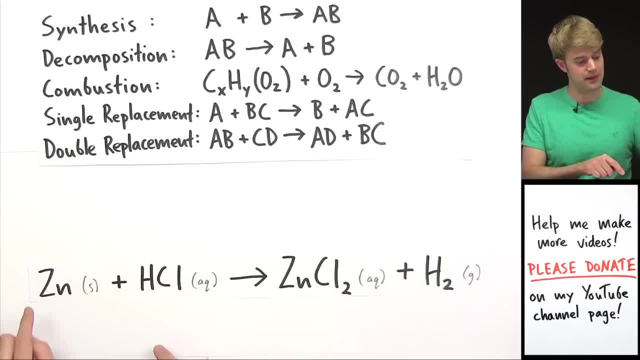 together. Hydrogen and chloride here are paired up, and then zinc by itself gives us hydrogen. So when we take the hydrogen out of the way and ends up pairing up with chloride, giving us hydrogen by itself. So when this happens, when an element on its own kicks out, 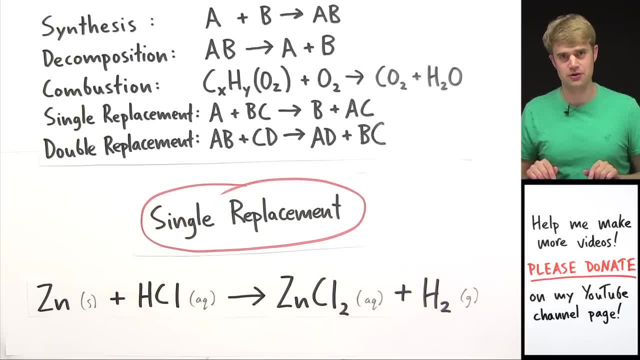 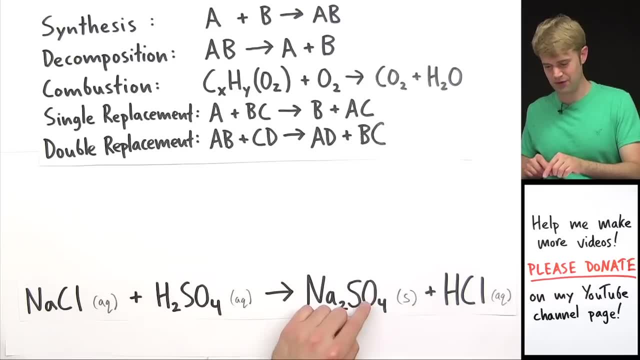 another element and takes its place in a pair. that is a great example of a single replacement reaction. Sodium chloride and H2SO4, known as sulfuric acid, come together to give us sodium sulfate and HCl hydrochloric acid. So what's happening here is that we have two pairs of two. 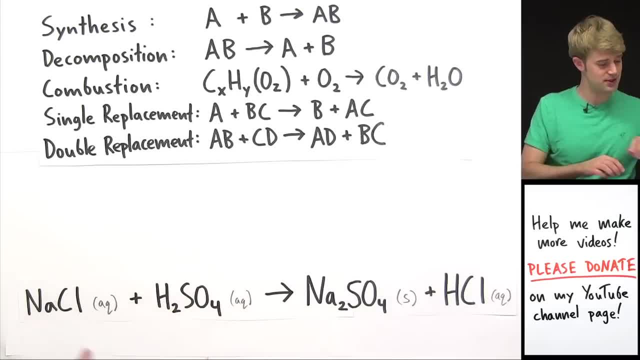 HCl and H and SO4. They switch places. So the Na that used to be paired up with the Cl ends up pairing up with the SO4, and the H that was initially paired up with the SO4 ends up paired up with the Cl. So this is an example here of a double replacement, A double replacement reaction. 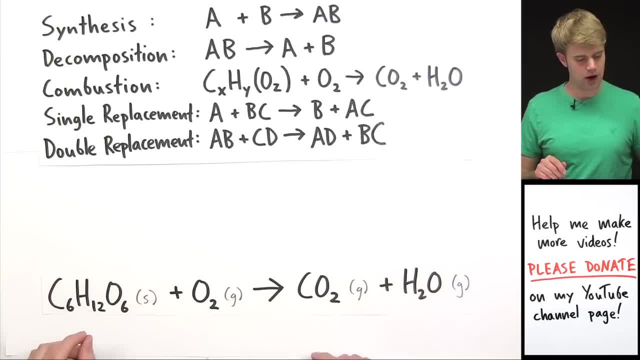 Okay, here's the last one, C6H12O6, which is the chemical formula for glucose. It's a sugar and food that you eat. Glucose is the chemical formula for glucose. It's a sugar and food that you eat. Glucose combines with oxygen to give us carbon dioxide and water. All right, this should look.